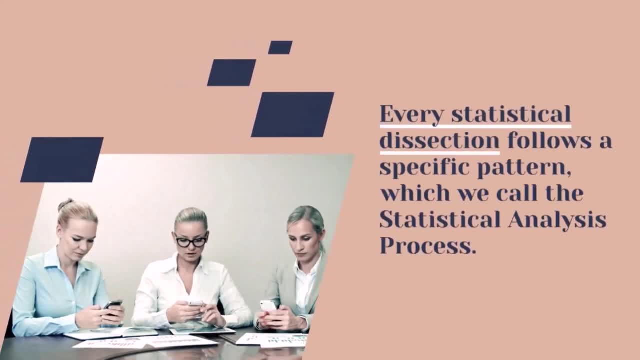 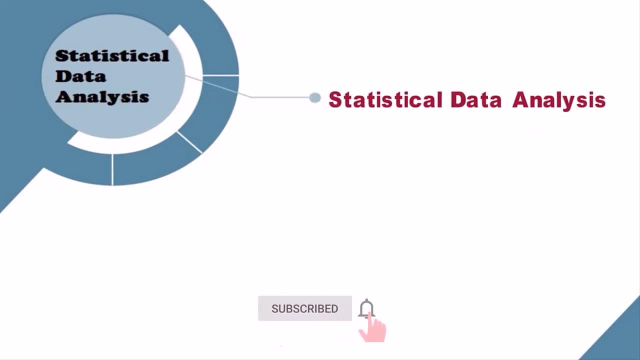 follows a specific pattern which we call the statistical analysis. Although there are many types of statistical data analysis, these two are the most common ones: 1. Descriptive statistics and 2. Inferential statistics. Let us discuss each in detail. 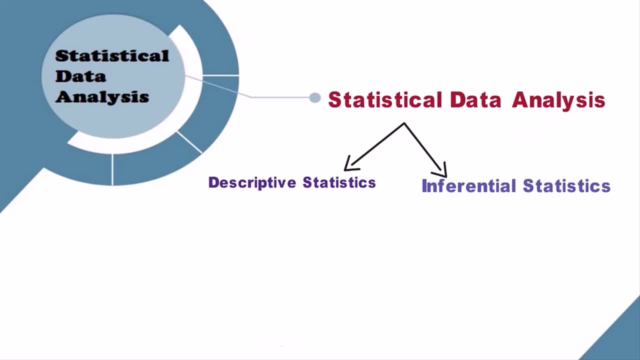 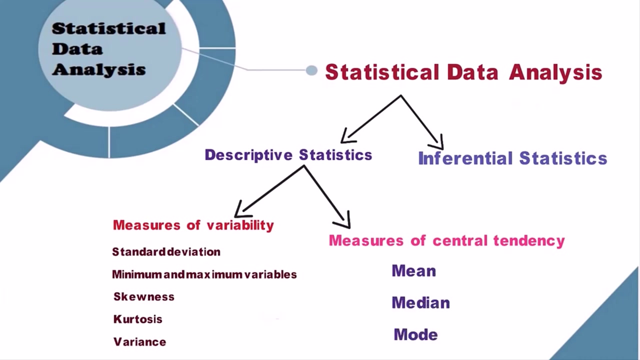 Descriptive statistics. It quantitatively summarizes the information in a significant way so that whoever is looking at it might detect relevant patterns instantly. Descriptive statistics are divided into measures of variability and measures of central tendency. Measures of variability consist of standard deviation, minimum and maximum variables, skewness, kurtosis and variance. 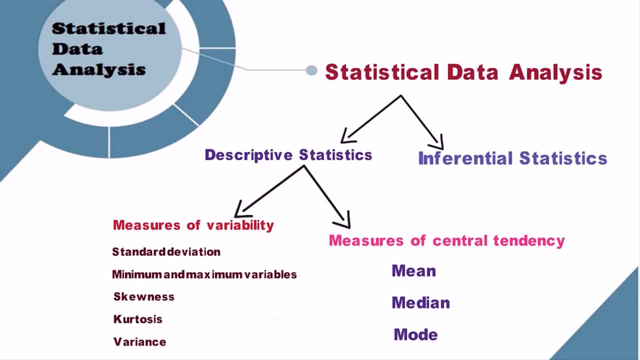 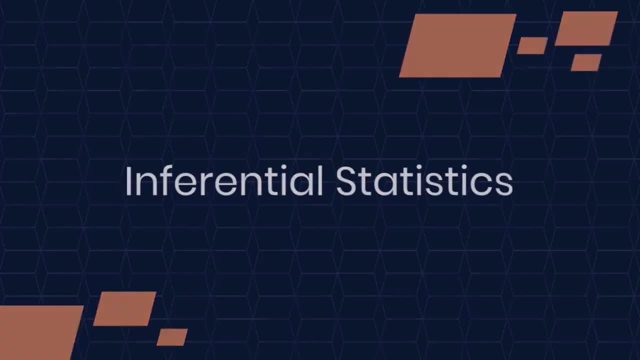 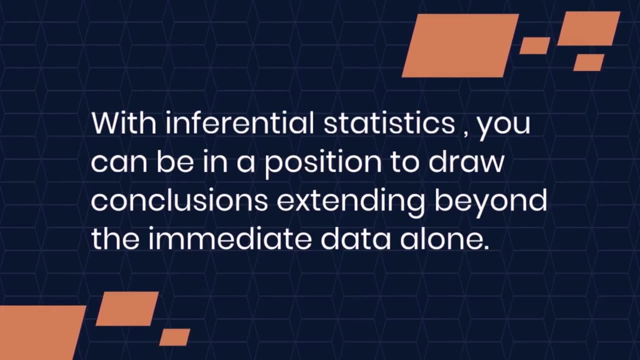 while measures of central tendency include the mean, median and mode Inferential statistics. With inferential statistics, you can be in a position to draw conclusions extending beyond the immediate data alone. We use this technique to infer from the sample data what the population might think or make judgments of the probability. 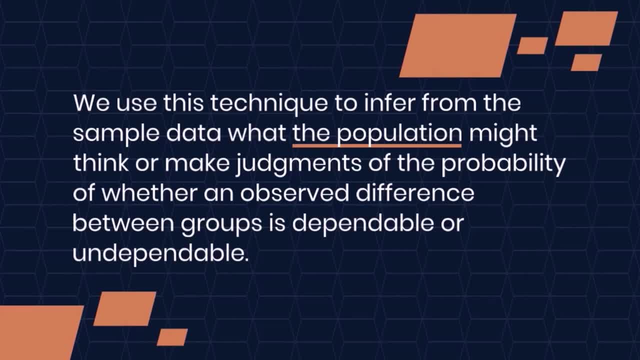 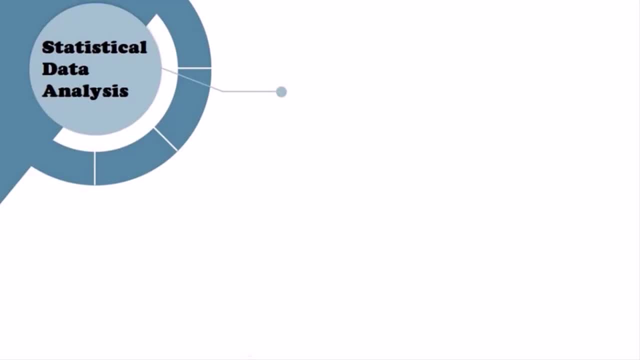 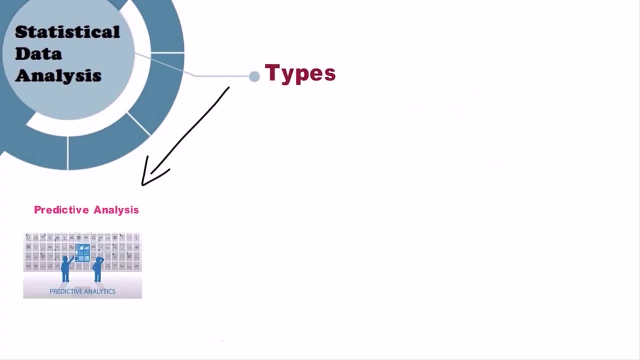 of whether an observed difference between groups is dependable or undependable. Undependable means it has happened by chance. Predictive analysis: Making predictions of future events based on current facts and figures. Prescriptive analysis: Examining data to find out the required actions for a particular situation. 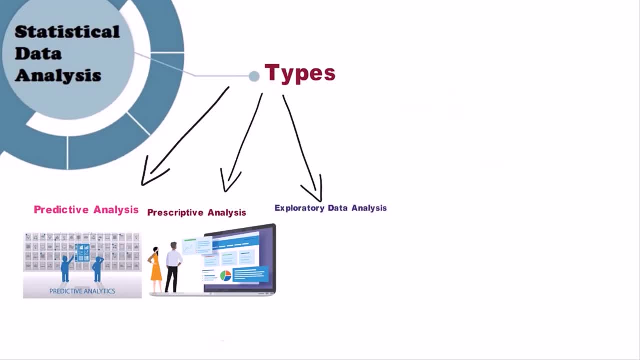 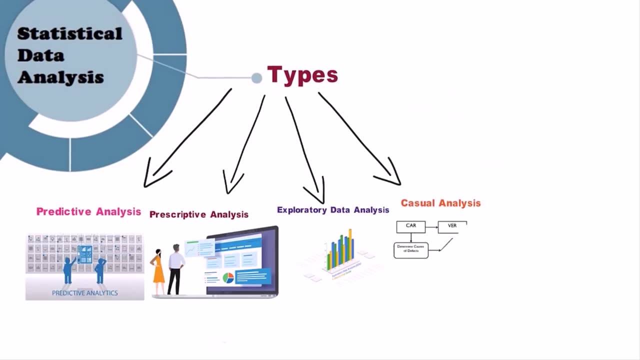 Exploratory data analysis: Previewing of data and assisting in getting key insights into it. Casual analysis, Determining the reasons behind why things appear in a certain way. Mechanistic analysis, Explaining how and why things happen, rather than how they will take place subsequently. 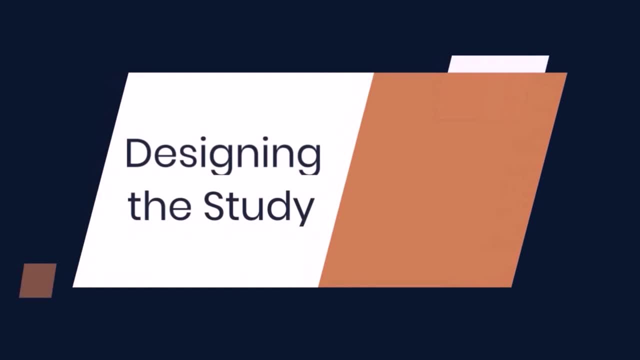 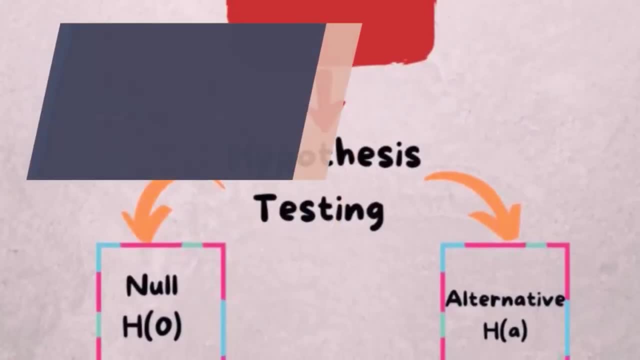 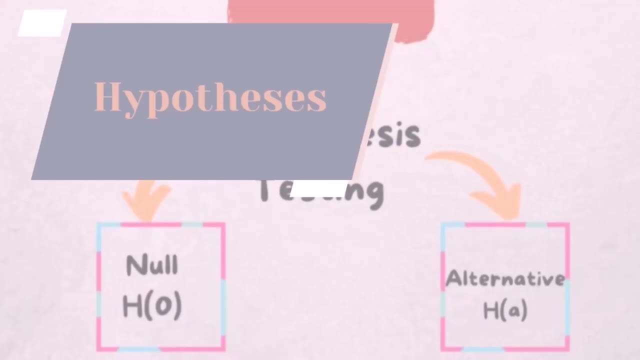 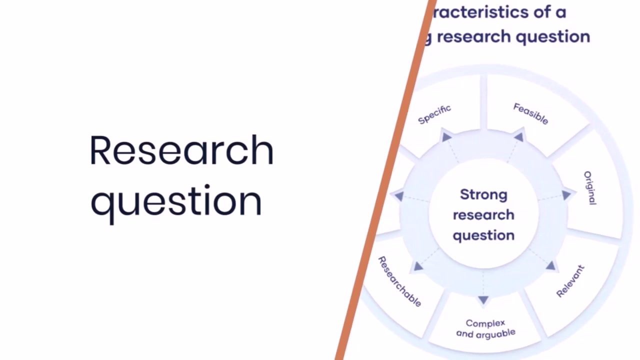 The statistical data analysis involves five steps. Step 1. Designing the study. the first and most crucial step in a scientific inquiry is stating a research question and looking for hypotheses to support it. Remember to find the relationship between variables within a population. when writing a statistical hypothesis, Every prediction you make can be either null or 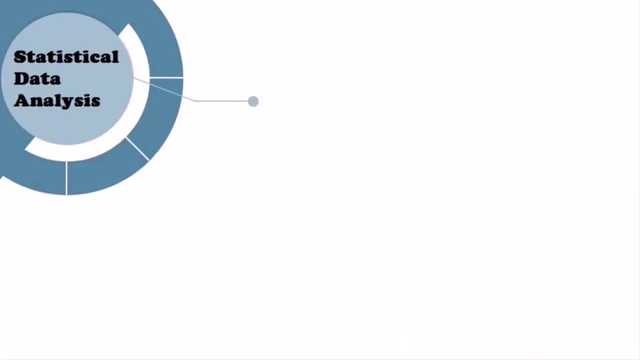 an alternative hypothesis. How to plan your research design. After deducing hypotheses for your research, the next step is planning your research design. It is basically coming up with the overall strategy for data analysis. There are three ways to design your research: 1. Descriptive. 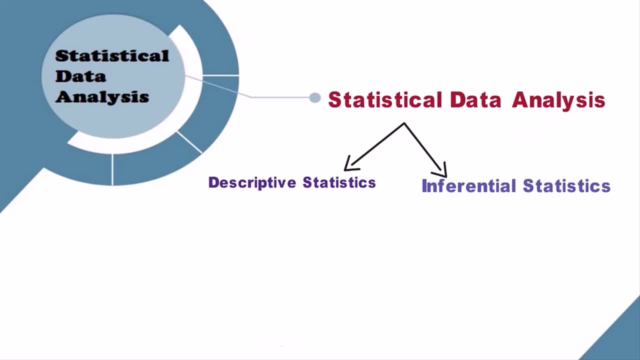 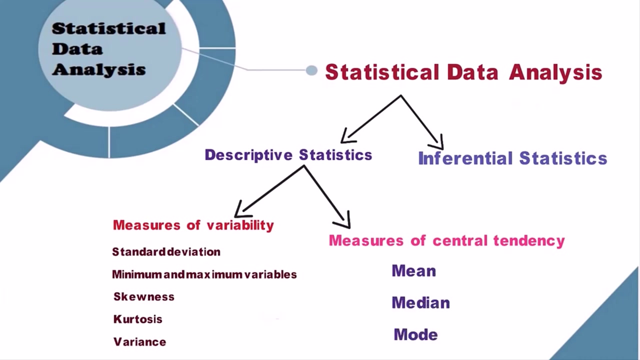 Descriptive statistics. It quantitatively summarizes the information in a significant way so that whoever is looking at it might detect relevant patterns instantly. Descriptive statistics are divided into measures of variability and measures of central tendency. Measures of variability consist of standard deviation, minimum and maximum variables, skewness, kurtosis and variance. 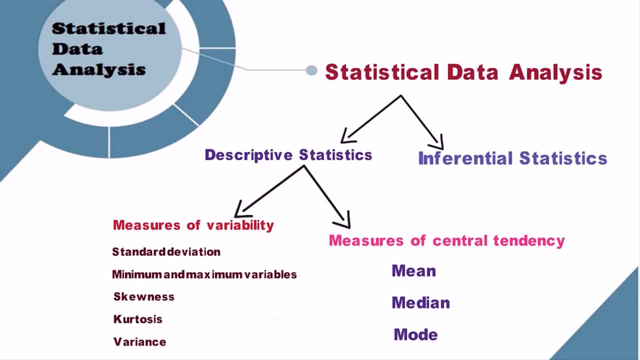 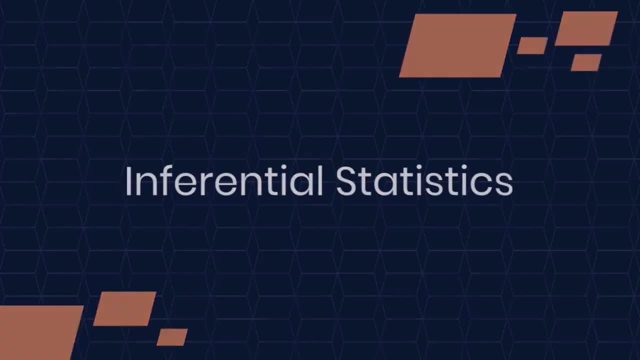 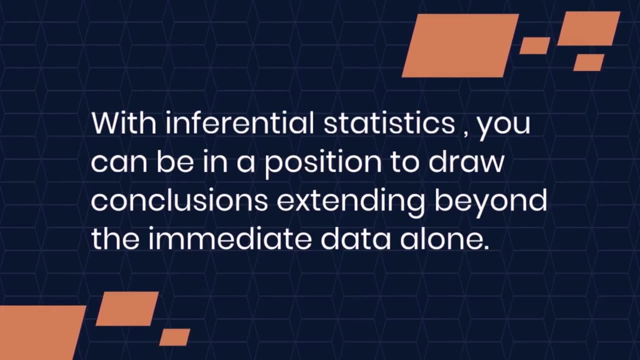 while measures of central tendency include the mean, median and mode Inferential statistics. With inferential statistics, you can be in a position to draw conclusions extending beyond the immediate data alone. We use this technique to infer from the sample data what the population might think or make judgments of the probability. 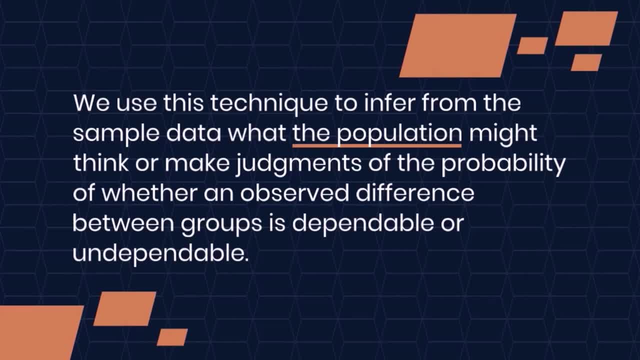 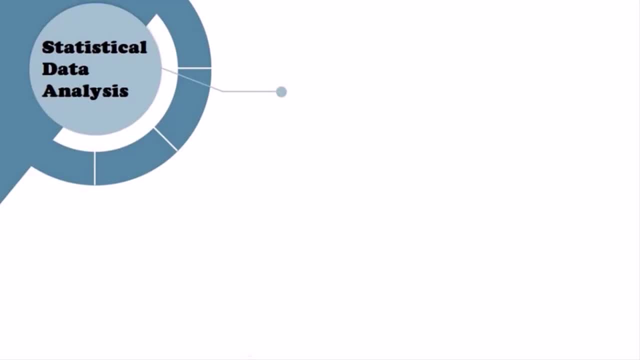 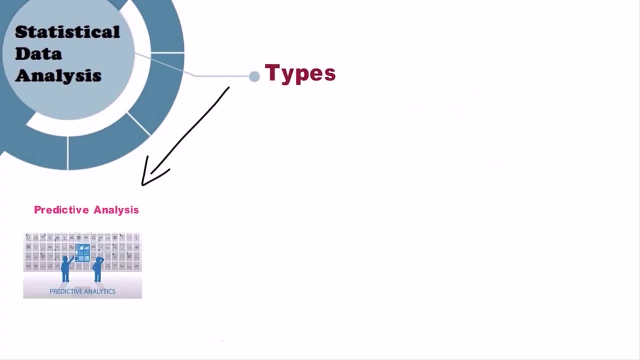 of whether an observed difference between groups is dependable or undependable. Undependable means it has happened by chance. Predictive analysis: Making predictions of future events based on current facts and figures. Prescriptive analysis: Examining data to find out the required actions for a particular situation. 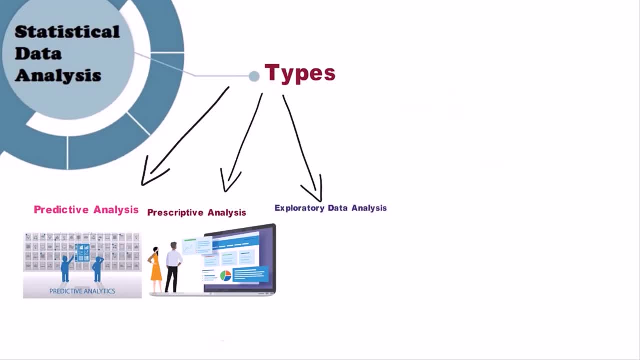 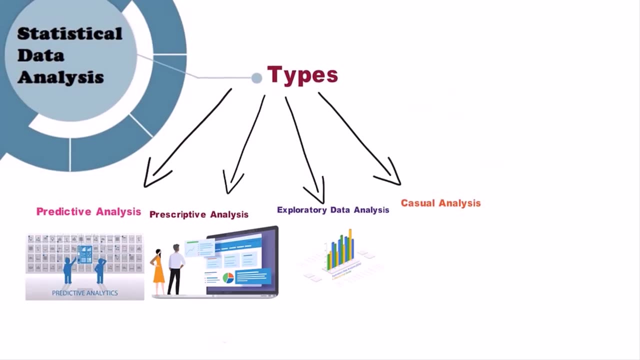 Exploratory data analysis: Previewing of data and assisting in getting key insights into it. Casual analysis, Determining the reasons behind why things appear in a certain way. Mechanistic analysis, Explaining how and why things happen, rather than how they will take place subsequently. 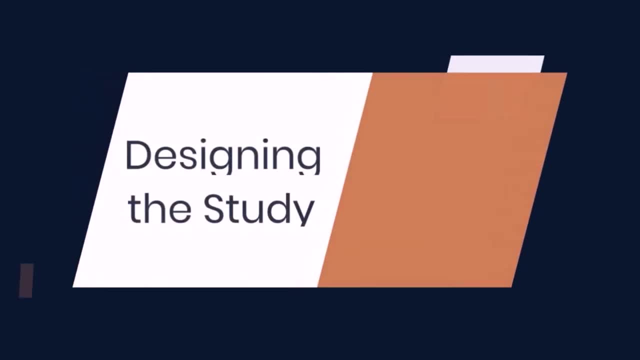 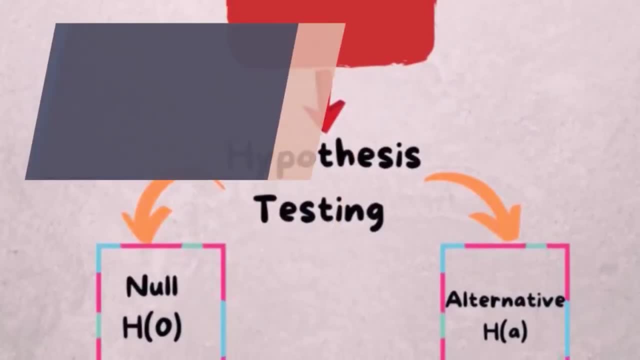 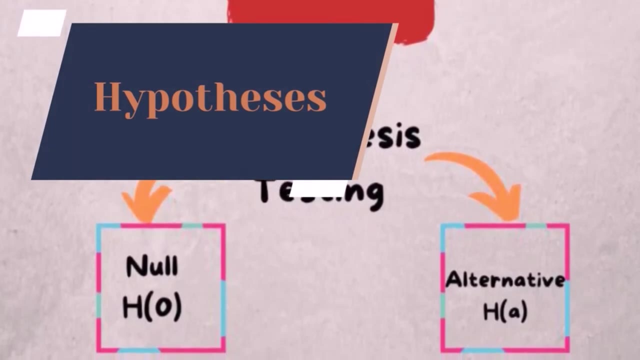 The statistical data analysis involves five steps. Step 1. Designing the study. the first step and most crucial step in a scientific inquiry is stating a research question and looking for hypotheses to support it. remember to find the relationship between variables within a population. 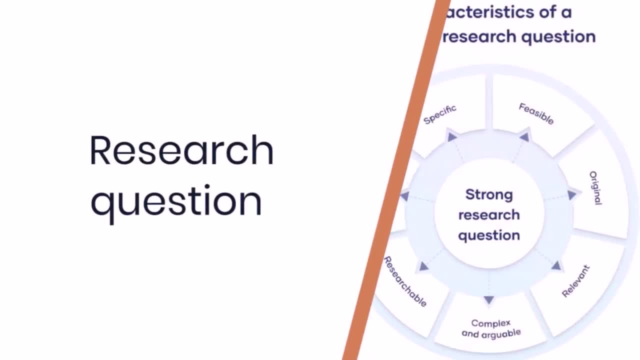 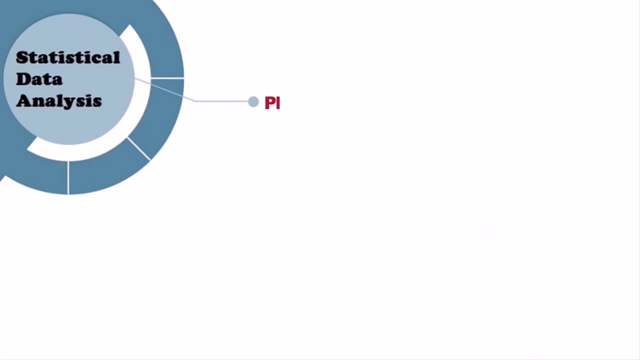 when writing a statistical hypothesis, every prediction you make can be either null or an alternative hypothesis. how to plan your research design. after deducing hypotheses for your research, the next step is planning your research design. it is basically coming up with the overall strategy for data analysis. there are three ways to design your research. one: descriptive design. 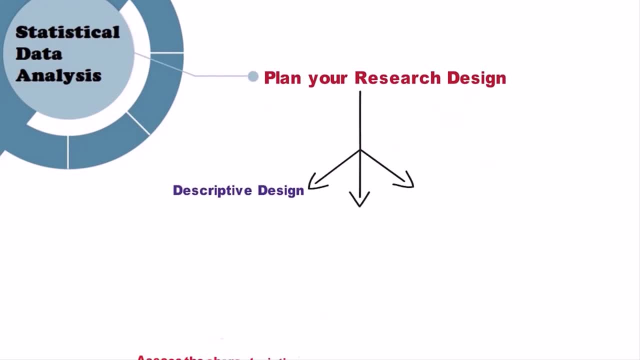 design. In a descriptive design, you can assess the characteristics of a population by using statistical tests and then construe inferences from sample data. 2. Correlational design, As the name suggests. with this design, you can assess the characteristics of a population by using 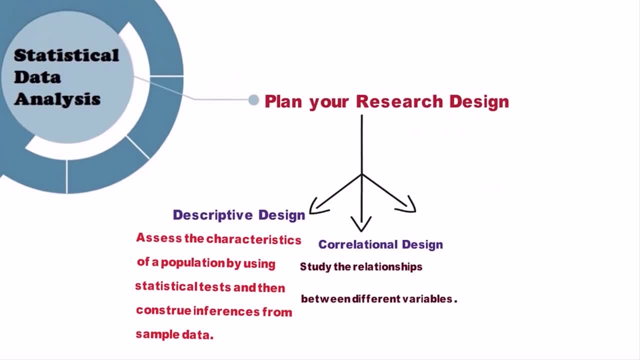 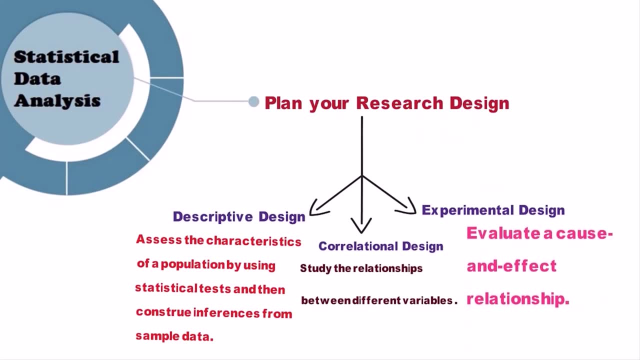 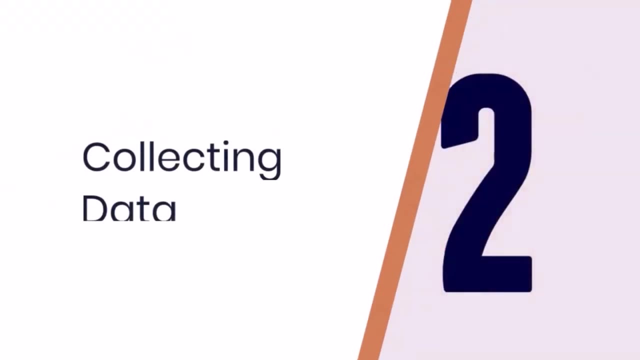 statistical tests, You can study the relationships between different variables. 3. Experimental design: Using statistical tests of regression and comparison, you can evaluate a cause and effect relationship. Step 2. Collecting data. Collecting data from a population is a challenging task. 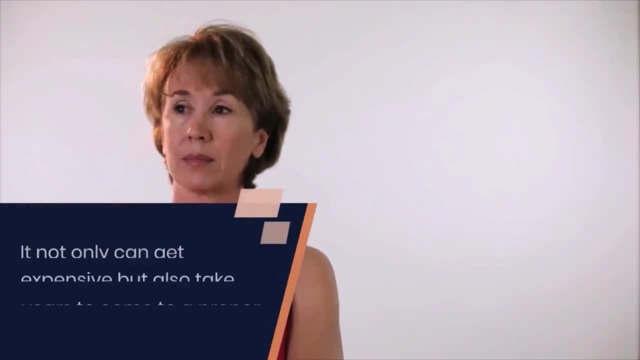 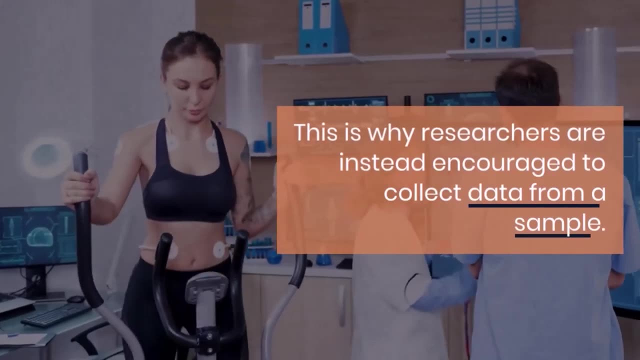 It not only can get expensive, but also take years to come to a proper conclusion. This is why researchers are instead interested in studying the relationship between different variables. Step 3. Sampling methods. Sampling methods in a statistical study refer to how we choose. 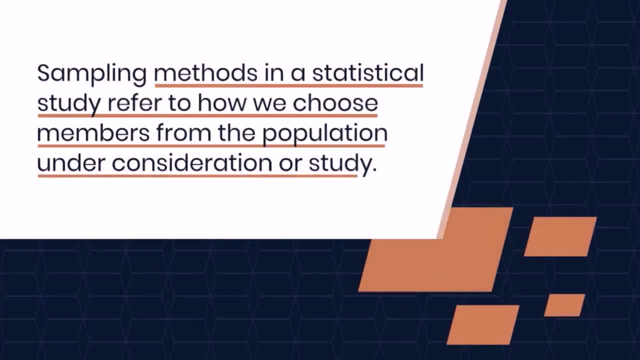 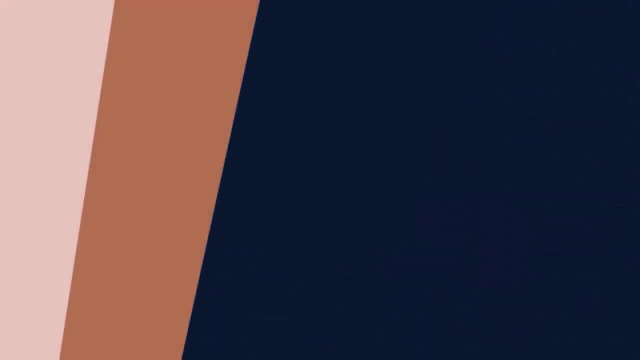 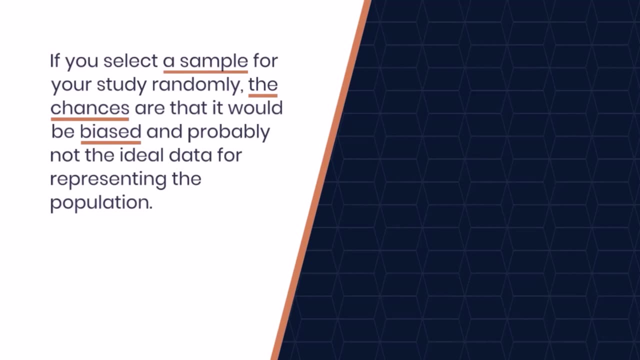 members from the population under consideration or study. If you select a sample for your study randomly, the chances are that it would be biased and probably not the ideal data for representing the population. This means there are reliable and non-reliable ways to select a sample. 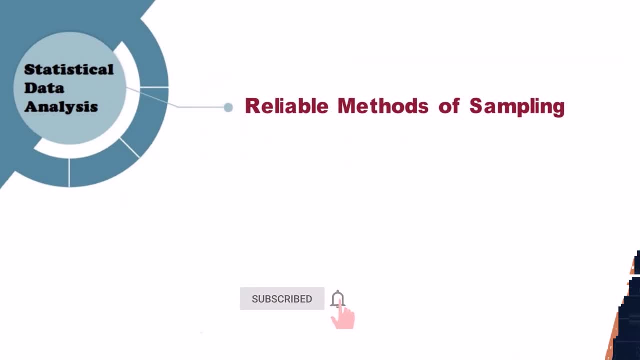 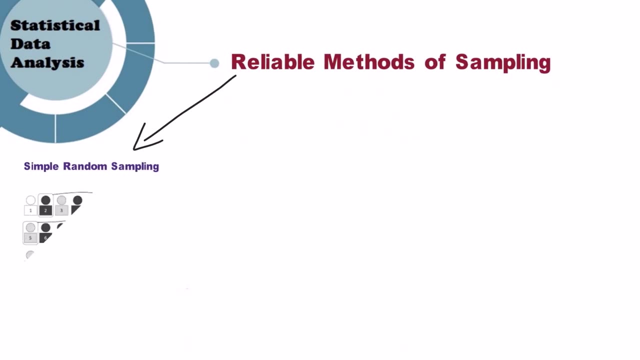 Reliable methods of sampling: Simple random sampling, A method where each member and set of members have an equal chance of being selected for the sample. Stratified random sampling: Population here is first split into groups, then members are selected from each group. Cluster random sampling: The population is divided into groups and members. 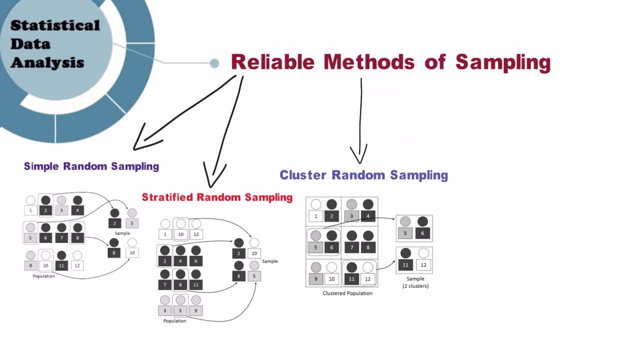 are randomly chosen from some groups. Systematic random sampling. Members are selected in order. the starting point is chosen by chance and every group is selected by chance. Every nth member is set for the sample. Non-reliable methods of sampling: Voluntary response sampling. 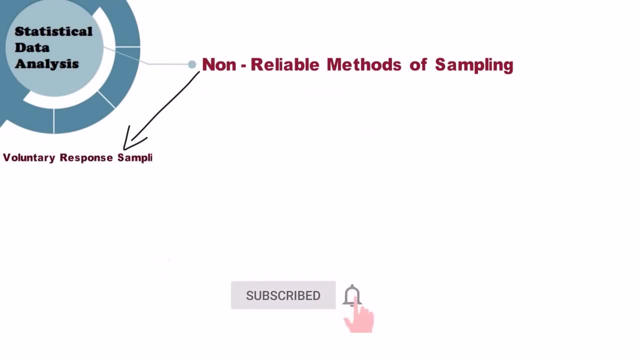 Choosing a sample by sending out a request for members of a population to join. Some might join and others might not respond. Convenient sampling: Selecting a sample readily available by chance. Here are a few important terms you need to know for conducting samples in statistics: Population standard deviation. 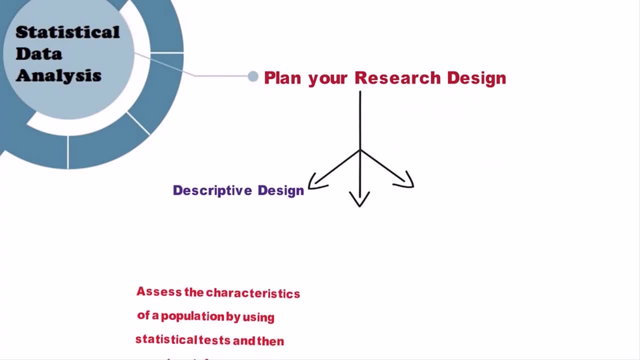 in a descriptive design, you can assess the characteristics of a population by using statistical tests and then construe inferences from sample data to correlational design, as the name suggests. with this design, you can study the results of the analysis available on the bar anymore the relationships between different variables. 3. experimental design using statistical tests. 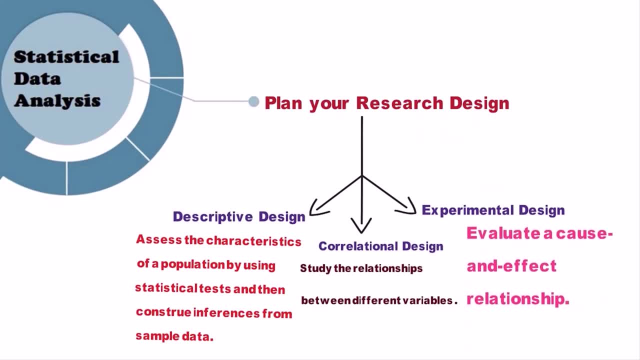 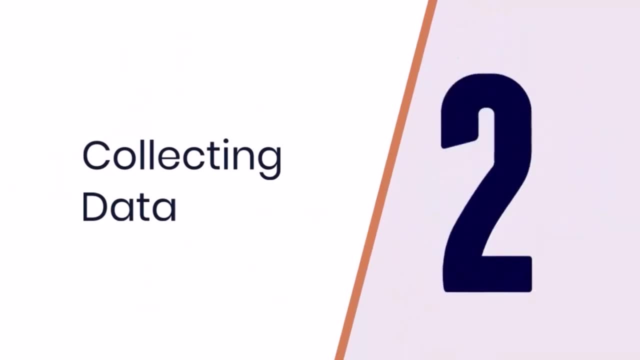 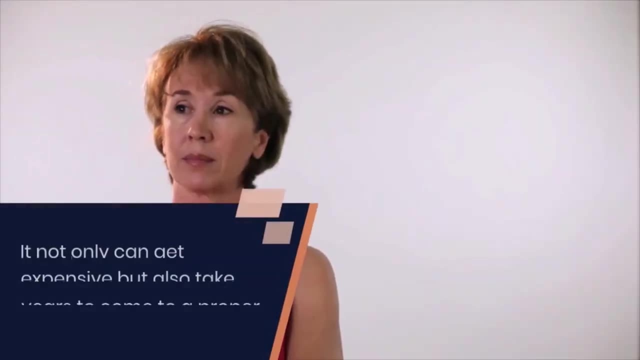 of regression and comparison, you can evaluate a cause and effect relationship. step 2: collecting data. collecting data from a population is a challenging task. it not only can get expensive, but also take years to come to a proper conclusion. this is why researchers are instead encouraged to collect data from a sample. 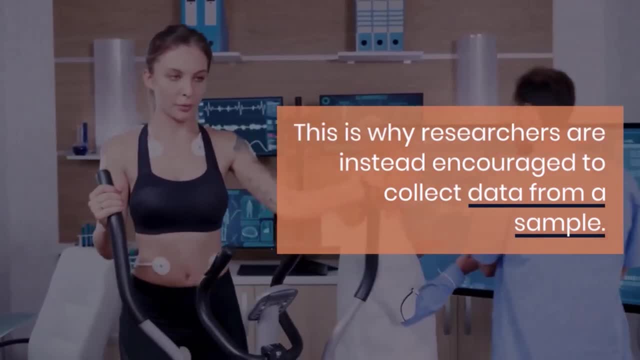 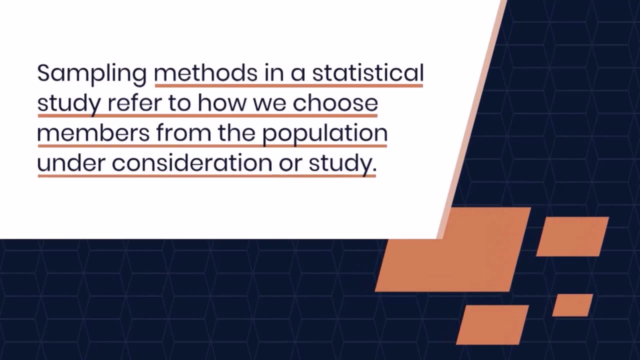 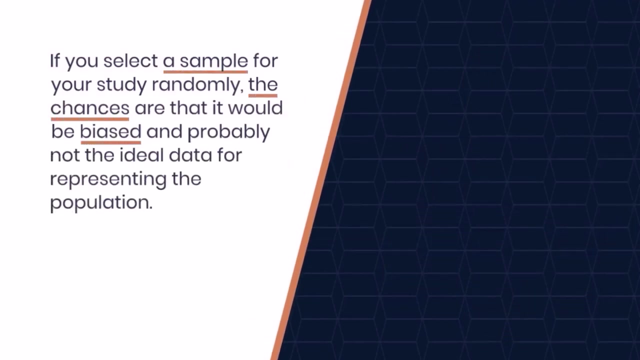 sampling methods in a statistical study refer to how we choose members from the population under consideration or study. if you select a sample for your study randomly, the chances are that it would be biased and probably not the ideal data for representing the population. this means there are reliable and non-reliable ways to select a sample. 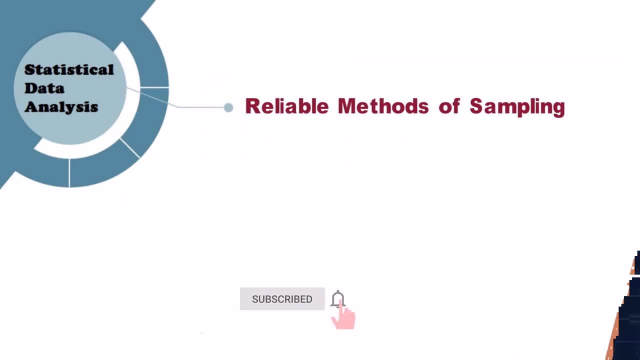 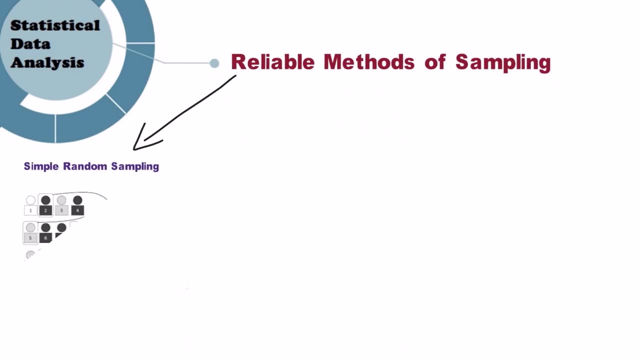 reliable methods of sampling: simple random sampling: a method where each member and set of members have an equal chance of being selected for the sample. stratified random sampling: population here is first split into groups. then members are selected from each group. cluster random sampling: the population is divided into. 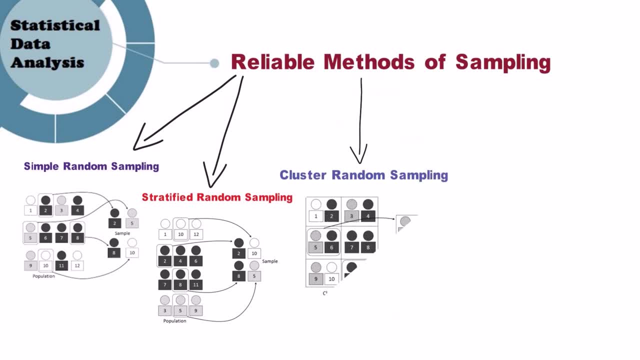 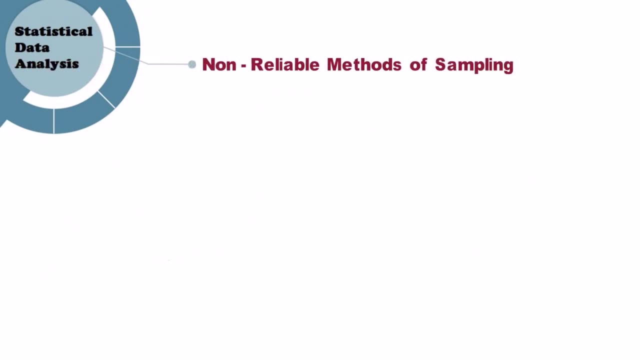 groups and members are randomly chosen from some groups. systematic random sampling. members are selected in order. the starting point of the sampling is determined by the number of members selected in order. the starting point is chosen by chance and every nth member is set for the sample. non-reliable methods of sampling: voluntary response sampling. choosing a sample by sending out a. 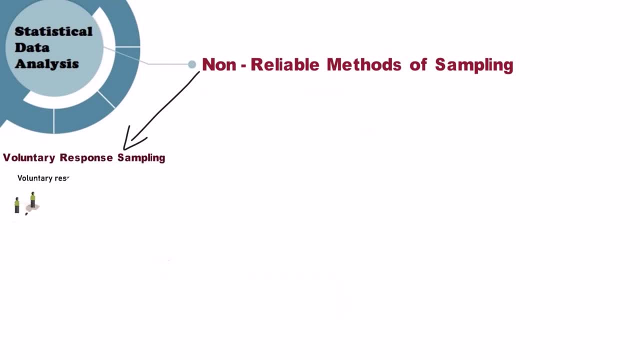 request for members of a population to join. some might join and others might not respond. convenient sampling, selecting a sample readily available by chance: here are a few important terms you need to know for conducting samples in statistics: population standard deviation. estimated population parameter. on the basis of the previous study. 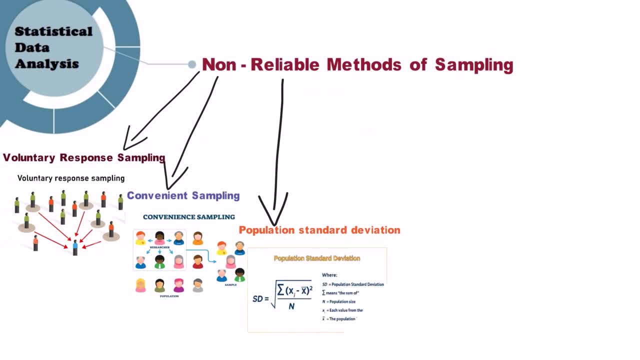 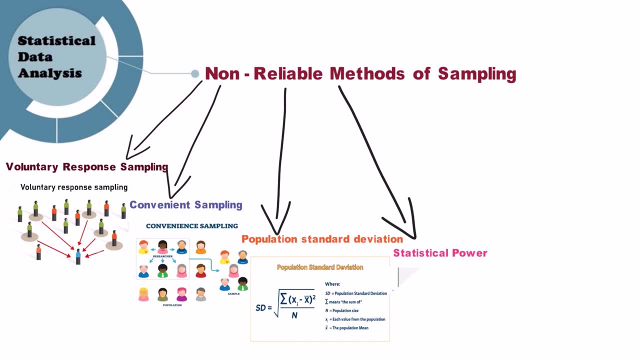 Amount of samples. Estimated population parameter on the basis of the previous study. Statistical power: The chances of your study detecting an effect of a certain size. Expected effect size. It is an indication of how large the expected findings of your research be. Significance: 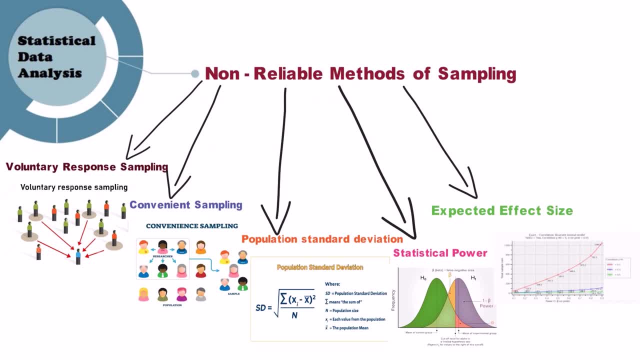 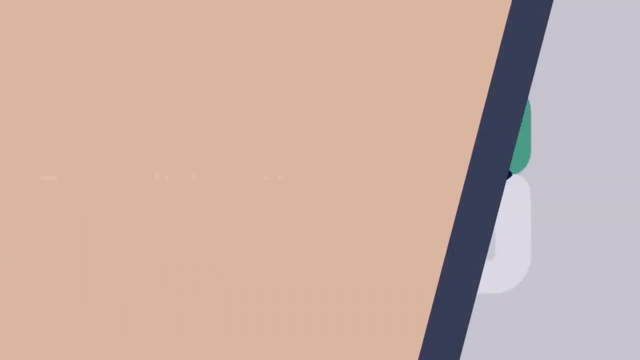 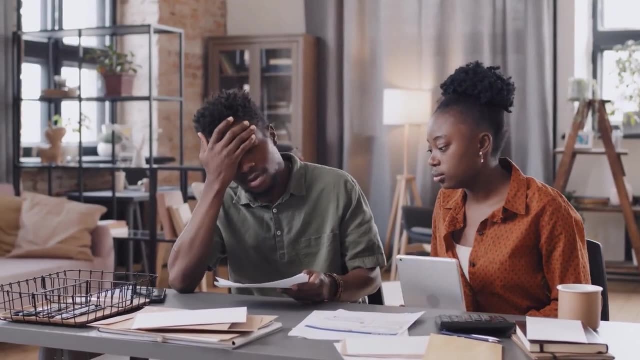 level Alpha, It is the risk of rejecting a true null hypothesis. Step 3. Describing the research data. Describing the data: Once you are done finalizing your samples, you are good to go with their inspection by calculating descriptive statistics, which. 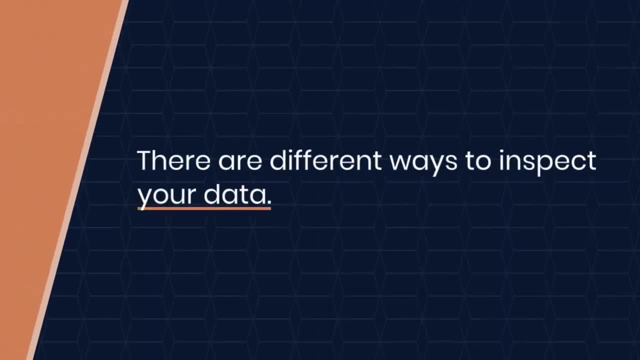 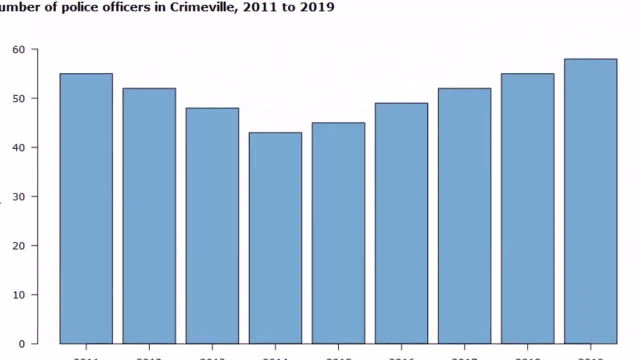 we discussed above. There are different ways to inspect your data: 1. By using a scatter plot to visualize the relationship between two or more variables. 2. A bar chart displaying data from key variables to view how the responses have been distributed. 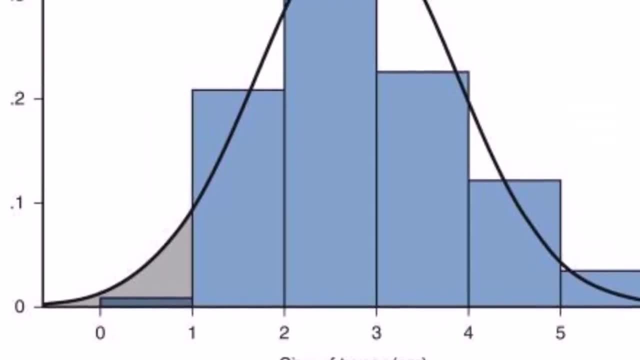 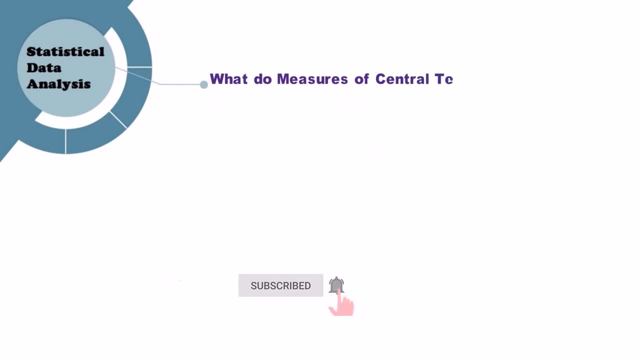 3. Via frequency distribution, where data from each variable can be organized. What do measures of central tendency do? Well, it precisely describes where most of the values lie in a data set. having said that, the three most heard and used measures of central tendency are: 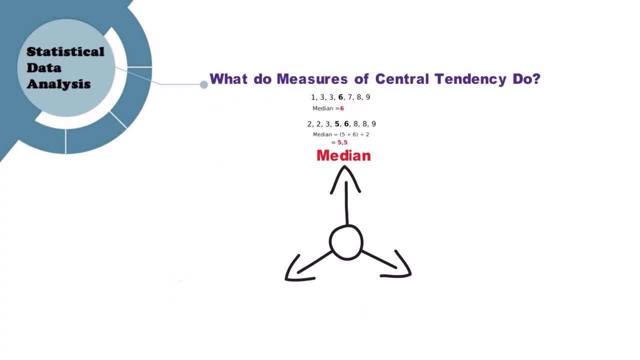 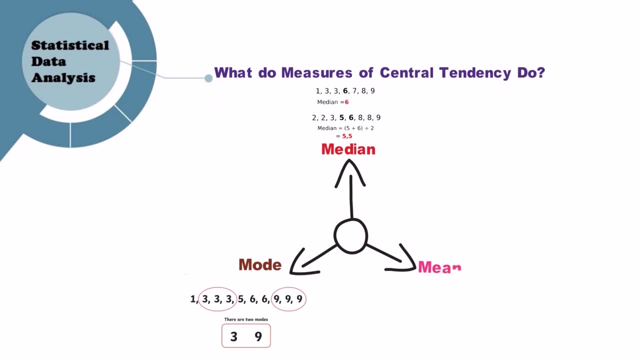 Median when considered from low to high. this is the value in the exact center Mode. mode is the most wanted or popular response. in the data set Mean. you calculate the mean by simply adding all the values and dividing by the total number. 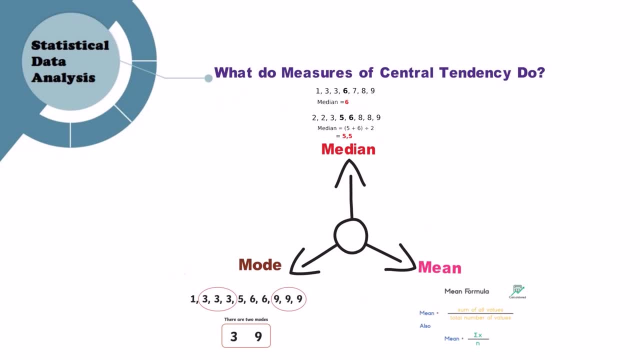 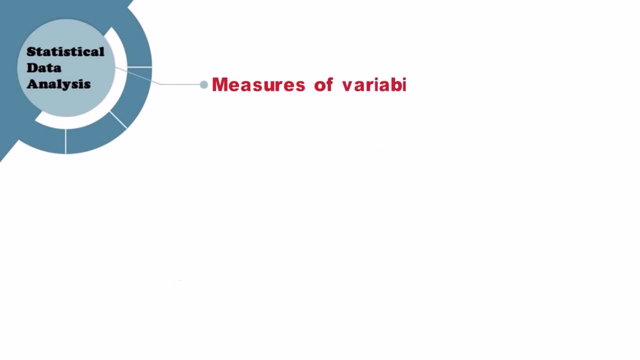 Coming to how you can calculate the- which is equally important- Measures of variability. Measures of variability give you an idea of how to spread out or dispersed values in a data set. The four most common ones you must know about are Standard deviation, the average distance between different values in your data set, and the 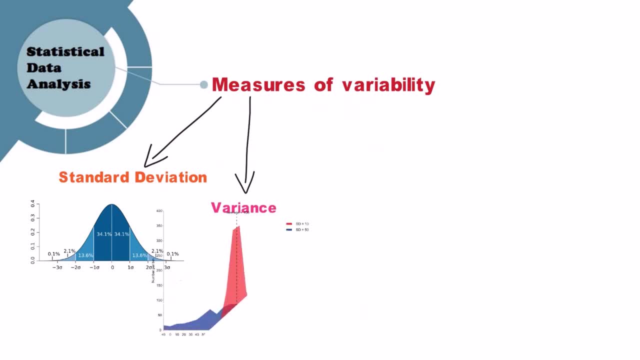 mean Variance. variance is the square of the standard deviation Range. the range is the highest value subtracted from the data set's minimum value. Interquartile range: interquartile range is the highest value minus lowest of the data. 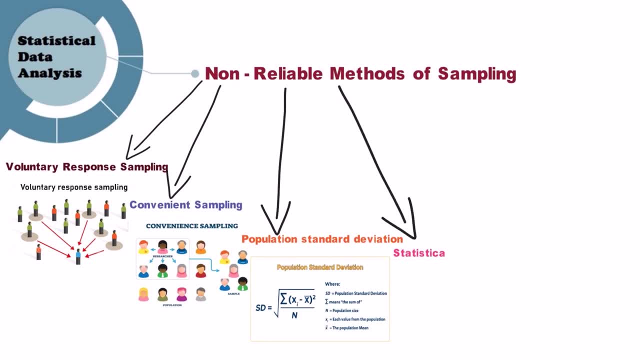 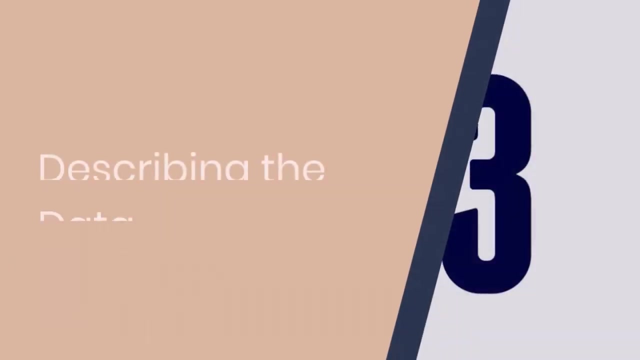 statistical power: the chances of your study detecting an effect of a certain size. expected effect size: it is an indication of how large the expected findings of your research be. significance level alpha: it is the risk of rejecting a true null hypothesis. step 3: describing the data once you are done finalizing your samples. 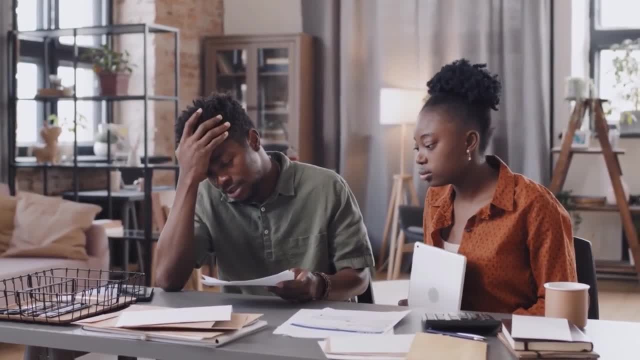 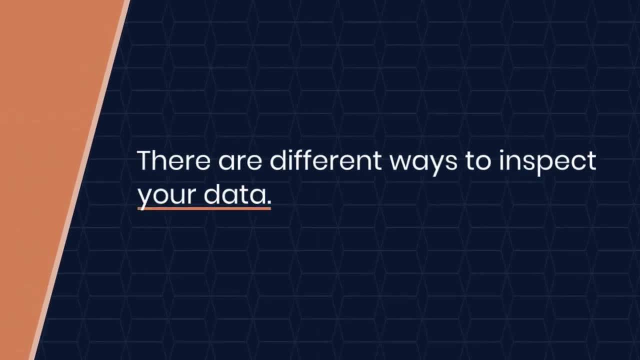 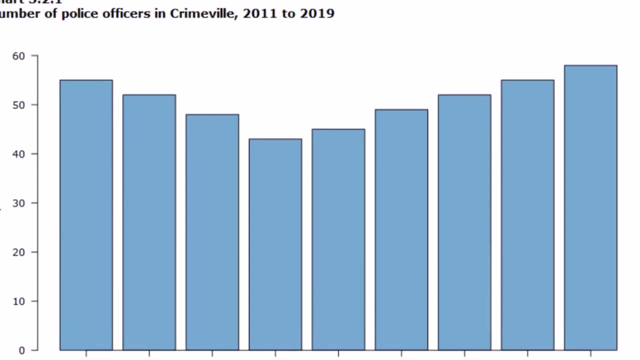 you are good to go with their inspection by calculating descriptive statistics, which we discussed above. there are different ways to inspect your data. one, by using a scatter plot to visualize the relationship between two or more variables. two, a bar chart displaying data from key variables to view how the responses have been distributed. 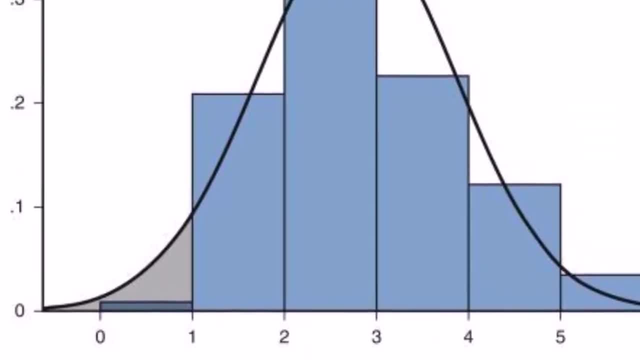 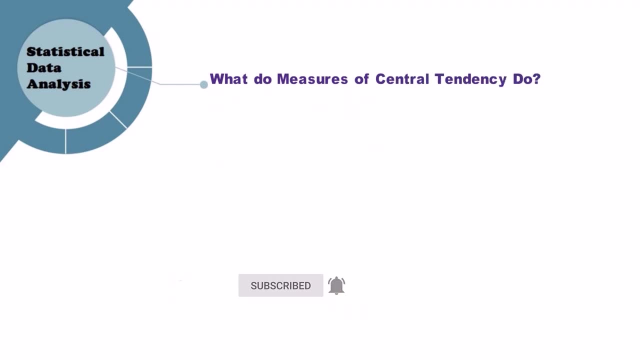 via frequency distribution, where data from each variable can be organized. what do measures of central tendency do? well, it precisely describes where most of the values lie in a data set. having said that, the three most heard and used measures of central tendency are median, when considered from low to high. this is the value in the exact center mode mode. 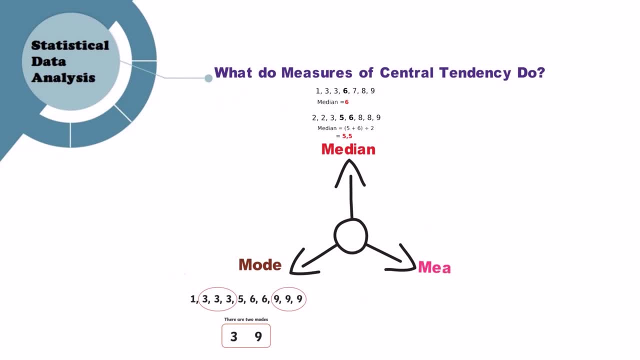 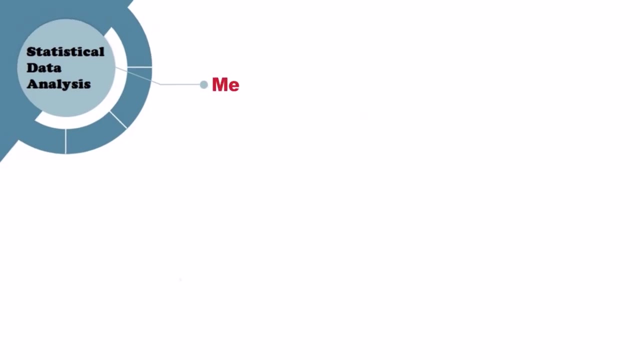 is the most wanted or popular response. in the data set Mean, you calculate the mean by simply adding all the values and dividing by the total number, Coming to how you can calculate the, which is equally important, Measures of variability. Measures of variability give you an idea of how to spread out or dispersed values in a 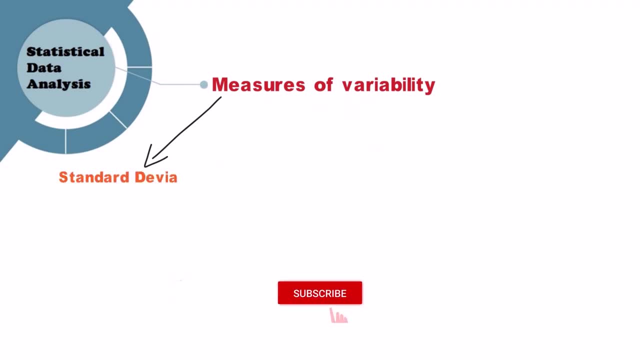 data set. The four most common ones you must know about are: standard deviation, the average distance between different values in your data set and the mean variance. variance is the square of the standard deviation range. the range is the highest value subtracted from the data. 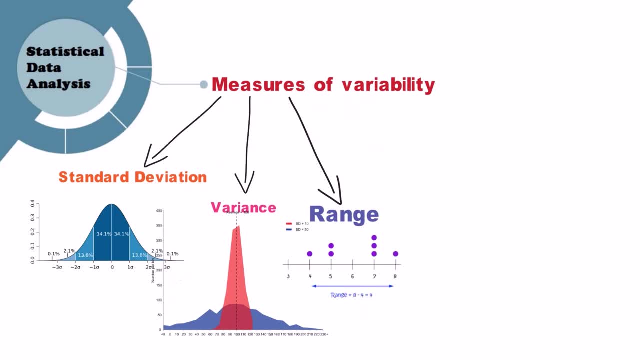 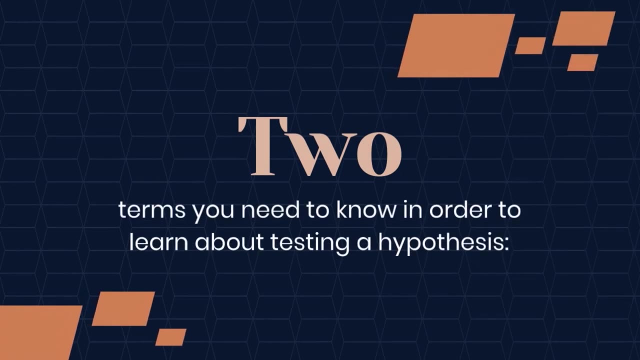 set's minimum value: interquartile range. interquartile range is the highest value minus lowest of the data set. Step four: testing your hypotheses. two terms you need to know in order to learn about testing a hypothesis Statistic: a number describing a sample.